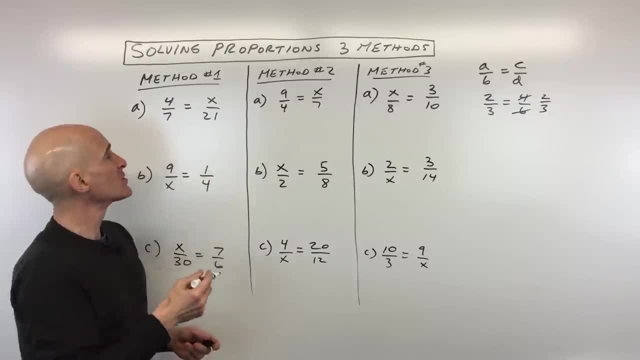 going to say: well, these fractions are equal to two-thirds. So we're going to say, well, these fractions are equal, right? So what I'm going to do is I'm going to multiply this denominator, see seven. I'm going to multiply it by three so that it gives me this denominator. 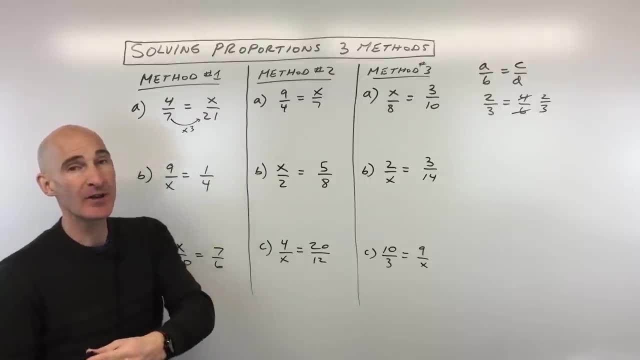 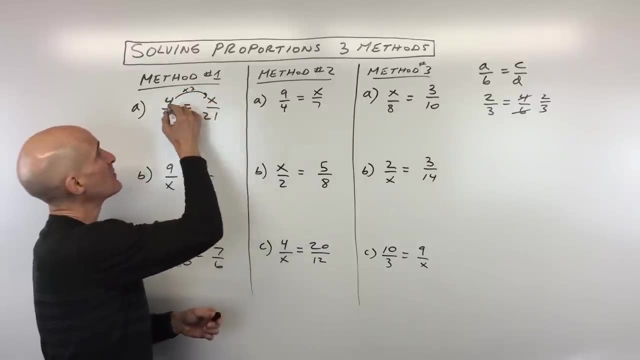 over here on the right 21.. But when you multiply the denominator by a quantity, you have to multiply the numerator by that same quantity. So I'm going to multiply the top also by three. So this is going to end up being four times three, which is 12, and that's what x is. That's the. 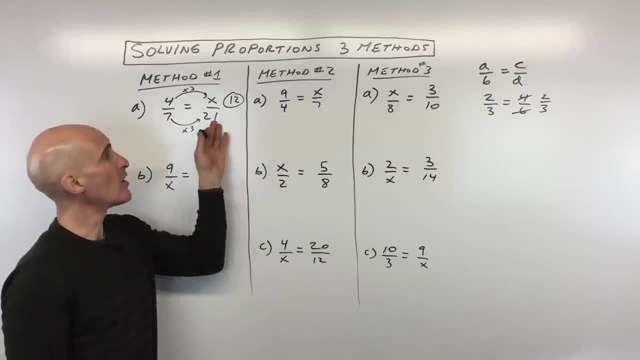 unknown quantity. Now, if you're not convinced, you can always reduce this 12 over 21.. You can see that three is equal to two-thirds, So I'm going to multiply the numerator by that same quantity. So three goes in here four times and three goes into 21 seven times. So you can see when we reduce. 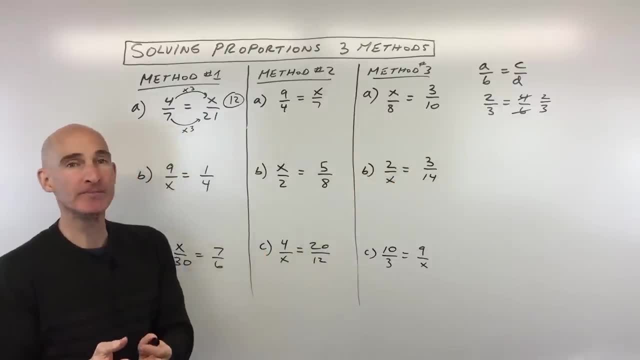 that fraction, just like we did at the beginning there, that they're equivalent, right? Okay, let's go to example number two. So here we've got: nine over x equals one over four. Okay, so now in this example I'm going to actually go from the right side to the left side. So I'm going to say, if I 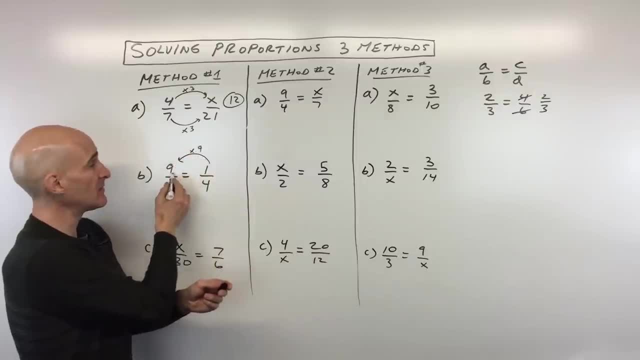 take one times nine, I get nine. But if I do that to the numerator of this fraction here on the right, I have to do the same thing to the denominator and multiply by nine. So I'm going to take nine. Well, four times nine is 36.. So that's our unknown quantity. x equals 36.. Again, you can. 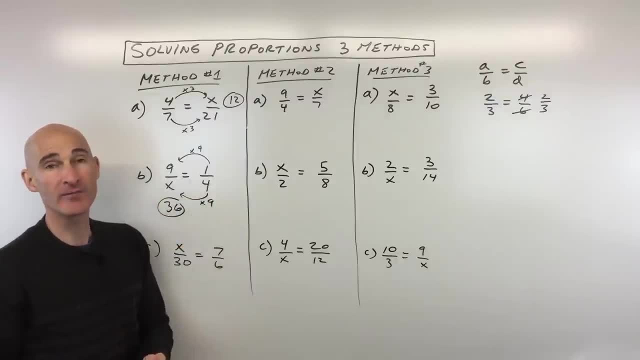 check: if you reduce 9, 36,, you're going to get one-fourth, So those are equivalent, Okay. last one, see if you can do this: one x divided by 30 equals seven divided by six. Okay, so here what? 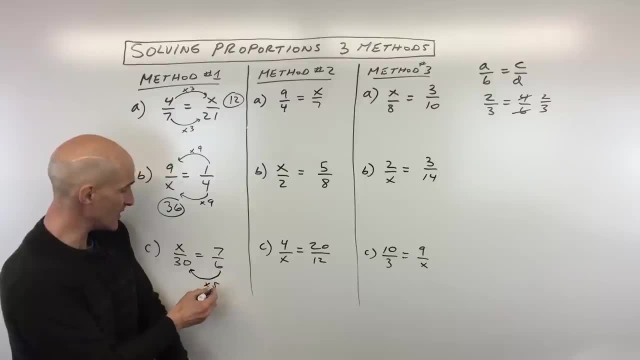 we're going to do is we're going to say: well, I know, six times five is 30. If I multiply the denominator by five, I have to multiply the numerator by five. So you can see, seven times five gives us 35. And again, if you reduce 35 over 30, it's going to be equivalent to 76.. Okay, so now? 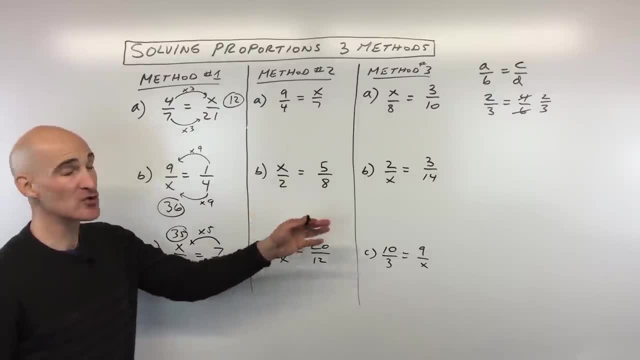 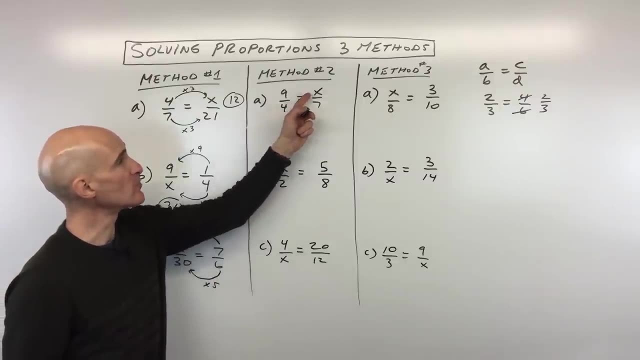 this is not the most favorite method, but stay with me. We're going to do two more different techniques, And you can, of course, use the one that you like the best. So method number two: we've got nine over four equals x over seven. Our goal is to find that variable, that unknown. 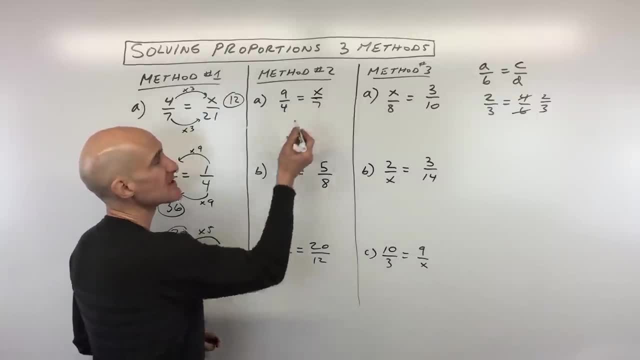 right. So what I'm going to do here, when you see this fraction bar, that's the same thing as division or dividing, right. So the opposite of dividing by seven would be to multiply by seven, Of course, if you do this to the right side of the equation. 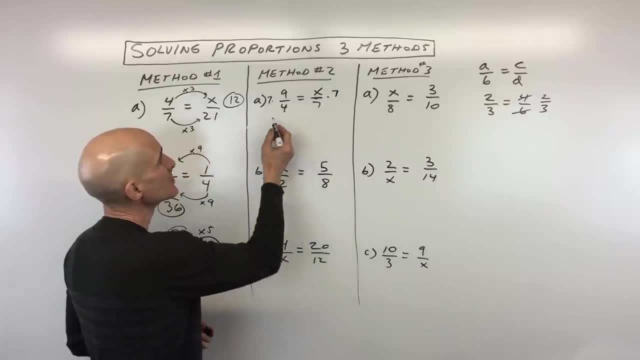 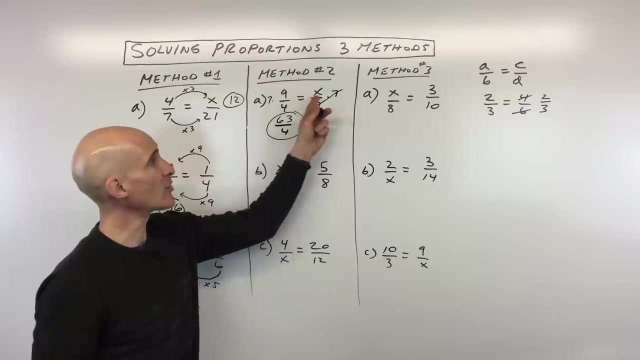 you have to do it to the left side to keep it balanced. So you can see this is going to end up being, let's see, seven times nine is 63 over four. these are going to cancel And that's our final result. So that's what x is. it didn't come out to a super nice number, But again, our goal is to 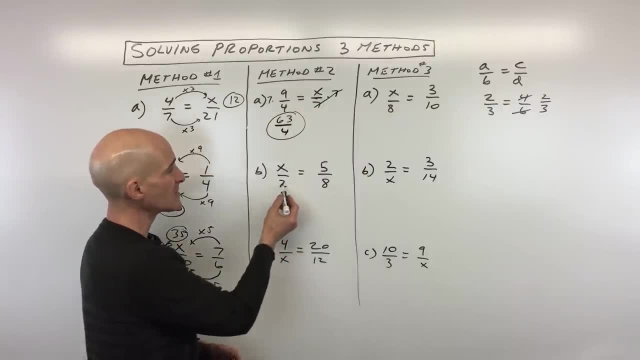 find out the unknown. Okay, let's look at example B here. So x divided by two equals five divided by eight. our goal is to find out the unknown. So let's look at example B here. So x divided by two equals five divided by eight. our goal is to find out the unknown. So let's look at example B here. So 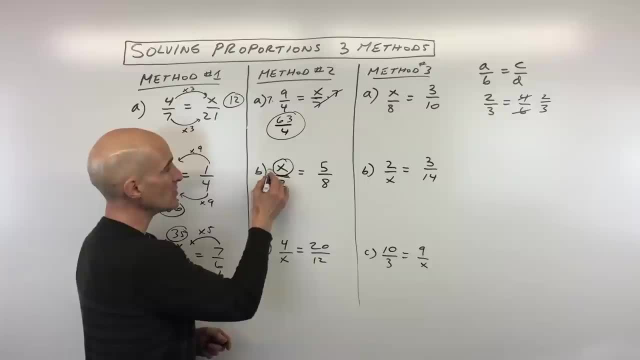 let's look at example B here. So x divided by two equals five divided by eight. our goal is to find out what this x is right. So the opposite of dividing by two is to multiply by two. that way those are going to cancel. We do that to the left, we have to do it to the right. now, two is the same as 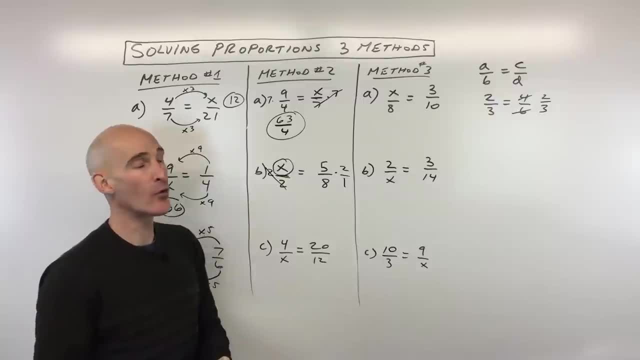 two over one. you can always write a whole number as a fraction by putting it over one, right? So you can see we're getting: five times two is 10.. Eight times one is eight, And we can reduce 10 over eight by dividing the top and bottom by two. 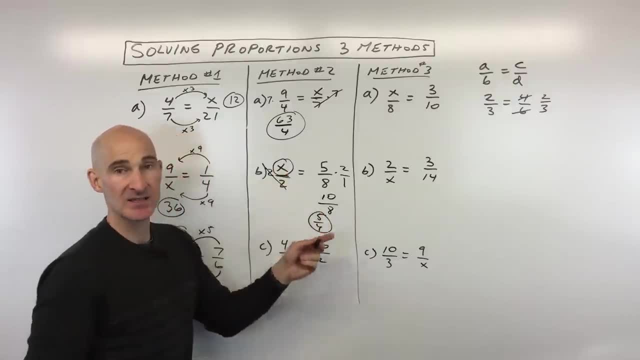 That's going to give us five fourths. Okay, so that's x in this example. okay, Last example of this type: 4 divided by x equals 20 divided by 12.. Okay, now this is a little bit different problem. 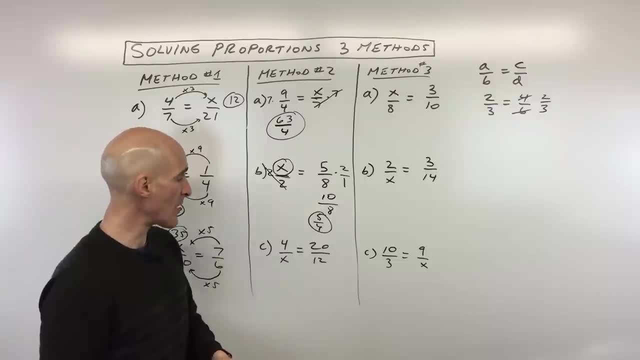 And because the variables in the denominator and one of the techniques or one of the properties of proportions, I should say, is that you can take the reciprocal of both sides of the equation. So if I flip this one over here on the left and make this x over 4,, 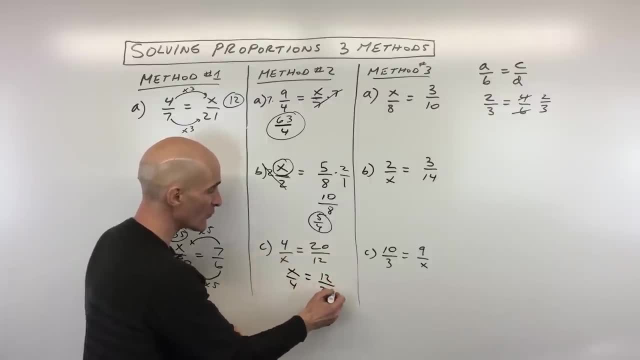 that's going to be the same thing as taking the reciprocal on the right, which is 12 over 20.. So now again, I'm going to do the opposite of dividing by 4.. I'm going to multiply both sides by 4, okay. 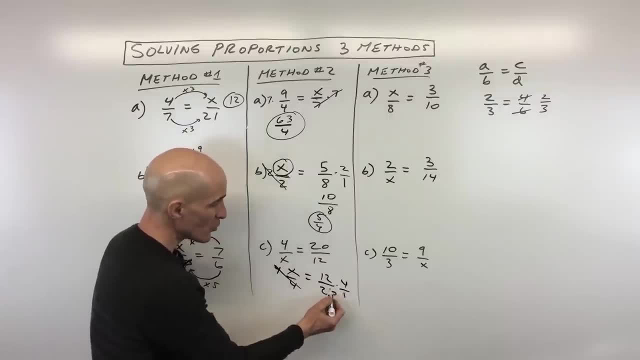 And what I'm going to do on this one is a little bit different. I'm going to do some cross-reducing, So I'm going to say 4 goes in here once, 4 goes into 25 times. So as long as you reduce numerator and denominator, you know. 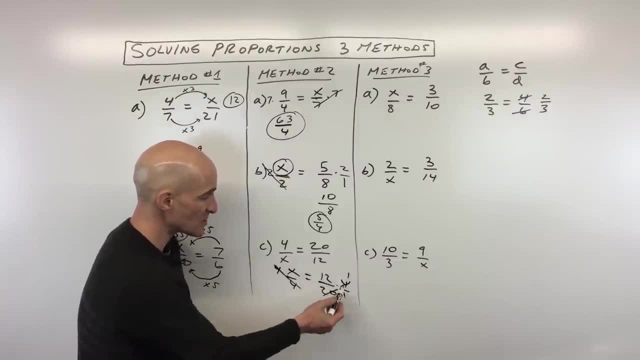 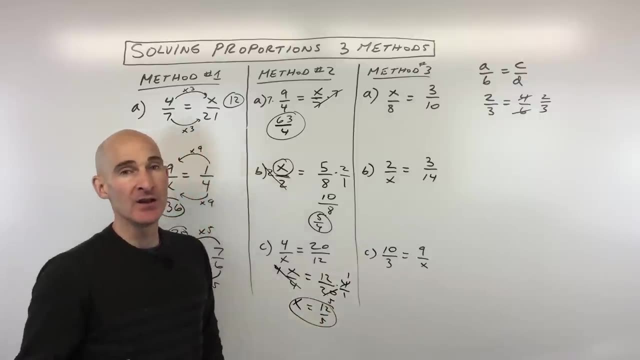 it doesn't matter whether it's in these two fractions or this fraction. this fraction you can reduce like that on the diagonal. And so here you can see, we're getting x equals 12 fifths. and you got it. So one last example, and this is probably the most favorite way of solving proportions: 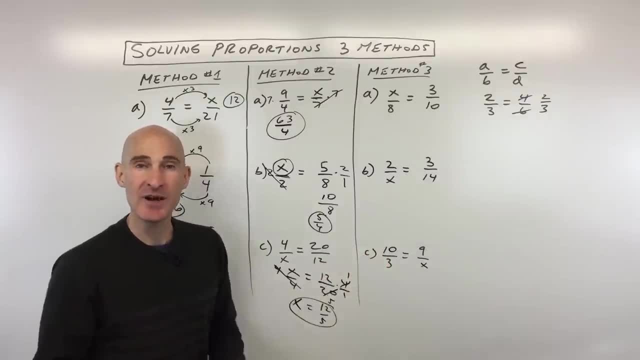 But before I do that, I just want to mention if you're enjoying my videos. you like my tutorials. I'd love to hear from you If you're enjoying my teaching style and you're learning Algebra 1, I've got a course called Learn Algebra 1,. 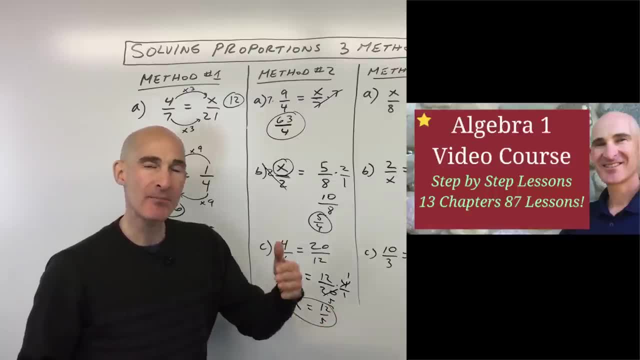 and I go through all the different concepts that are covered in that course step-by-step, with lots of examples, instruction, so that you can really grasp Algebra 1.. And check out that course. I'll have links to that. You can also check out the 13 free previews to see if it's a good fit for you. 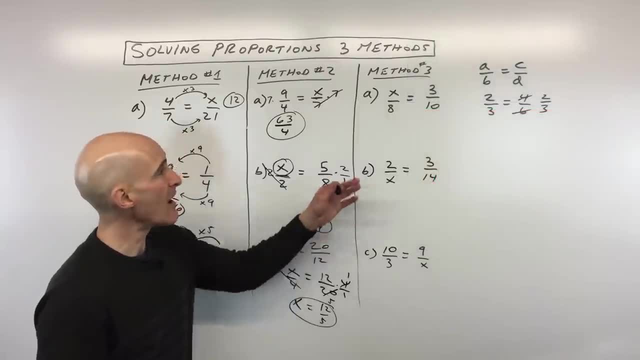 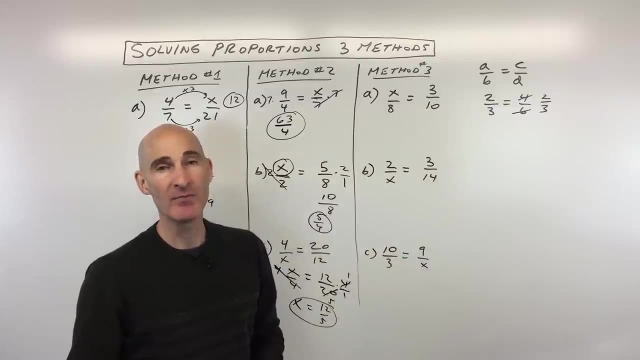 and pick up some pointers along the way as well. So my last method, method number 3, and that's that we're going to solve this by using the cross-reducing method, The cross-product method or the cross-multiplying method. 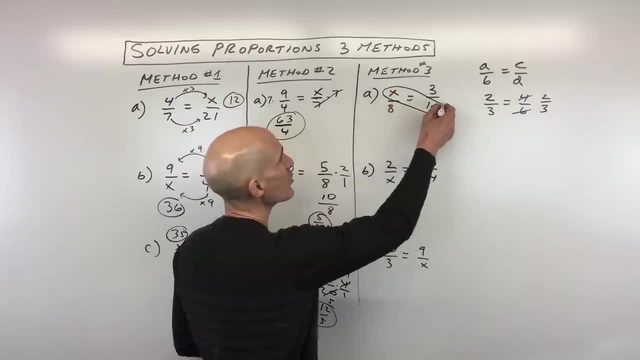 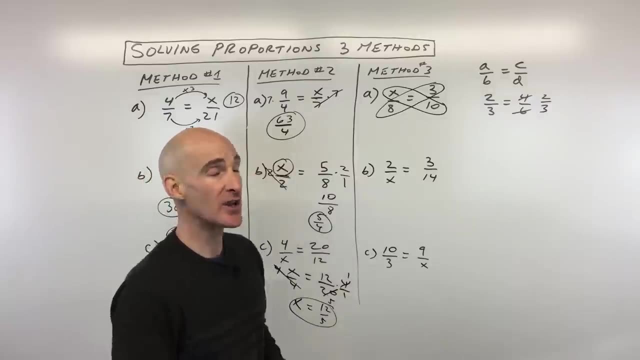 however, you want to say that, And the way this works is that this diagonal here multiplied together equals this diagonal here multiplied together, And what this does when you cross-multiply is it gets rid of the fractions, which a lot of times students don't like fractions. 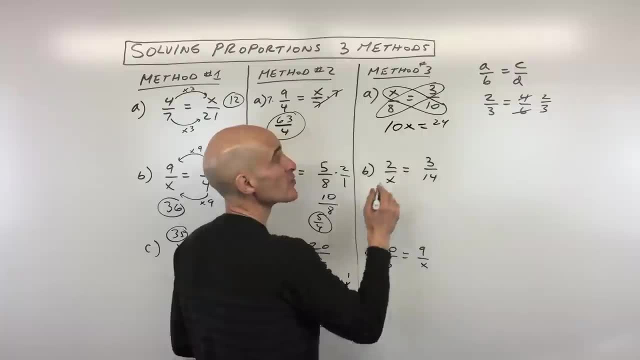 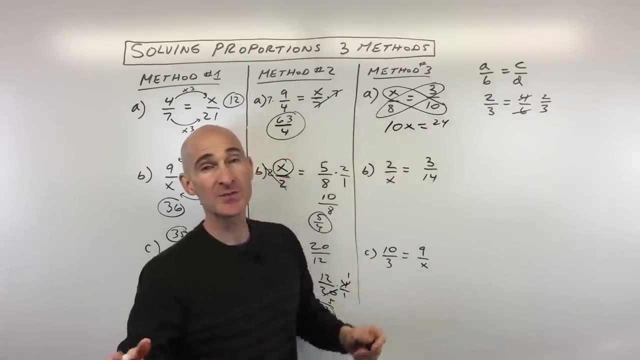 That might be your situation as well, but this gets rid of them for you. So basically, this diagonal multiplied together, 10 times x equals this diagonal multiplied together, which is 24.. Now some students ask me: does it matter if I put the 10x here? 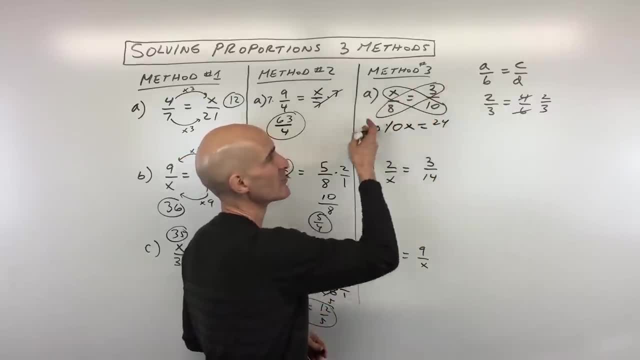 the 10x here. It doesn't matter, Just put the one diagonal on one side and then the other diagonal on the other side, right. And then the last step is: we're trying to solve for x, but because these are right next to each other, that means they're multiplied together. 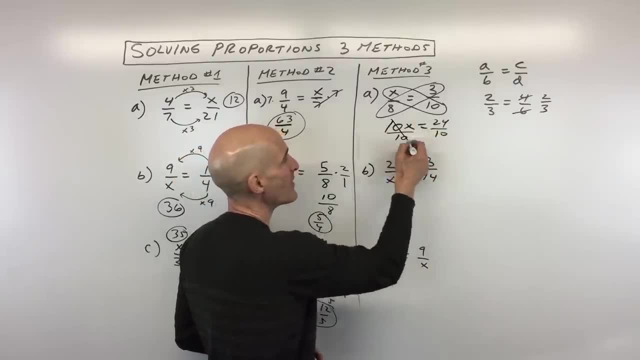 What's the opposite of multiplying by 10?? Of course it would be to divide by 10, right? So we've got: x equals 24 tenths and 10 goes into 24, let's see two times with four left over. so that's 2 and 4 tenths. 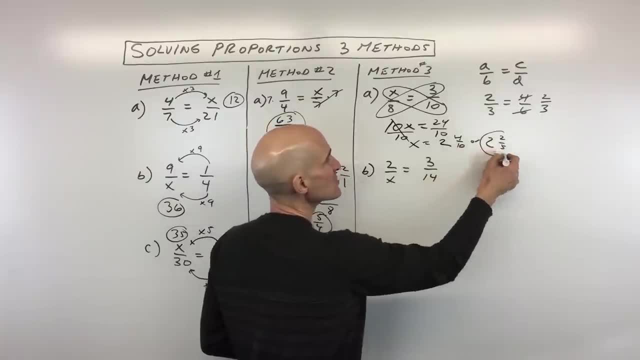 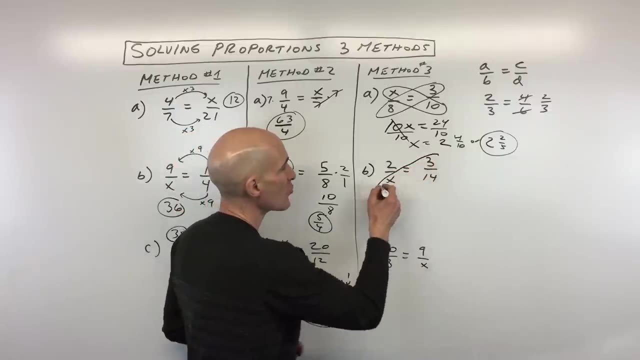 or 4 tenths. you can reduce to 2 fifths. so 2 and 2 fifths. Okay, see, if you can try these other two examples, we'll go through them, Okay. so here, what I'm going to do again is cross multiply. 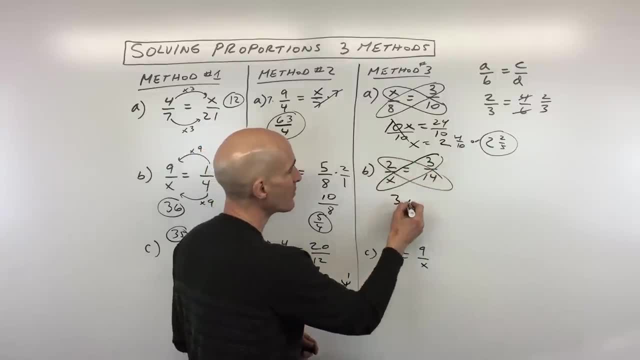 so that diagonal multiplied together equals that diagonal multiplied together. So we've got 3x equals 28,. divide both sides by 3, okay, and you can see. x equals 28 thirds and if you want, you can write it as a mixed number. 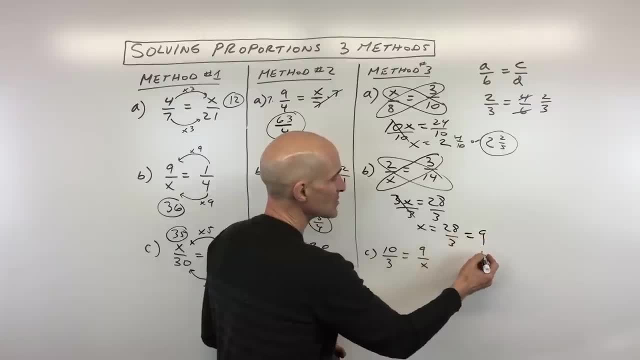 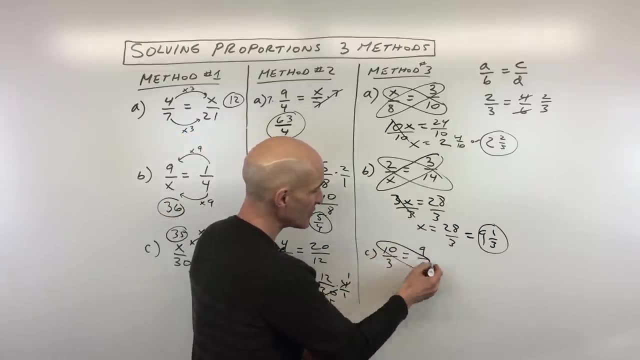 3 goes into 28. how many times? Let's see 9, that's 27 with one left over. so 9 and 1. third right. Okay, last one again: multiplying on the diagonals: right.